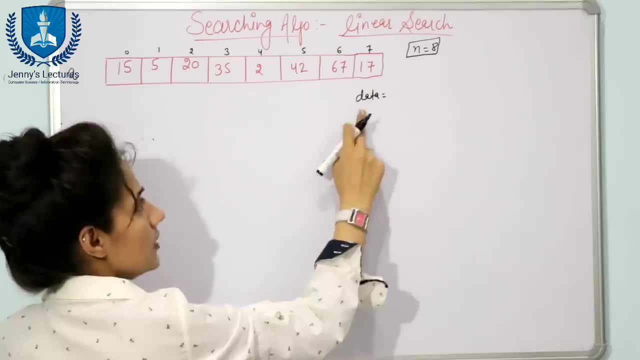 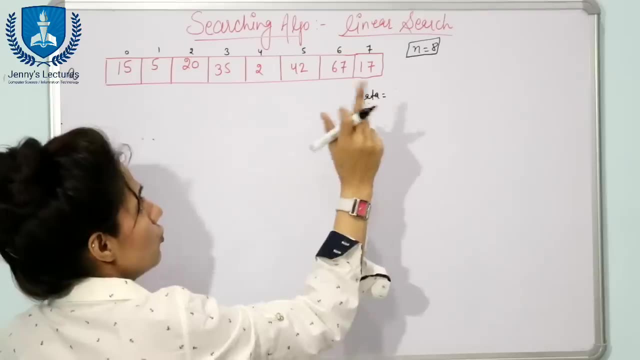 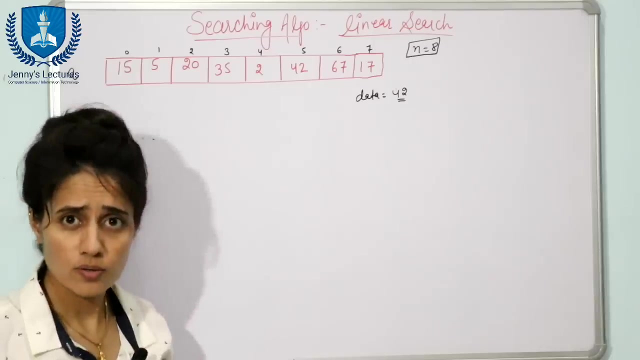 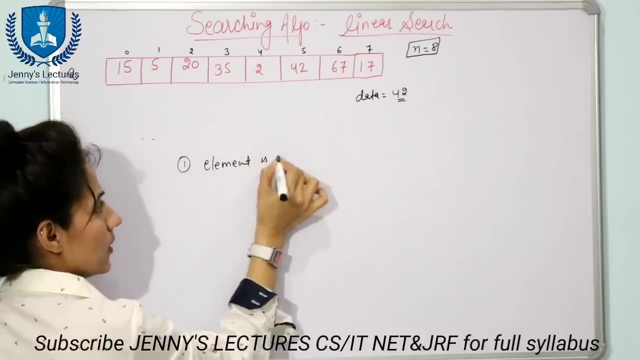 and value of this data or key, or you can take any variable. I am going to take here data, a variable data. Suppose you want to search 42.. You want to search: is 42 present in this array or not? Now, here, two cases are there. One is element is present in the list and second is not present. 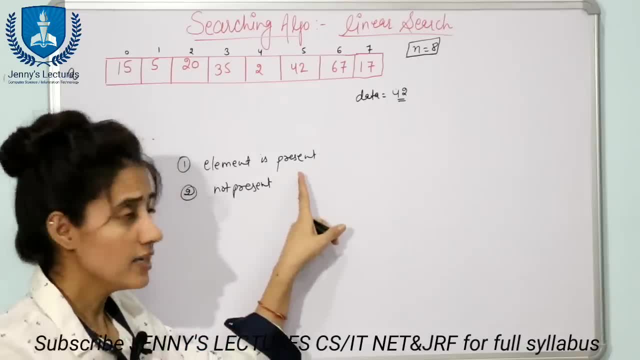 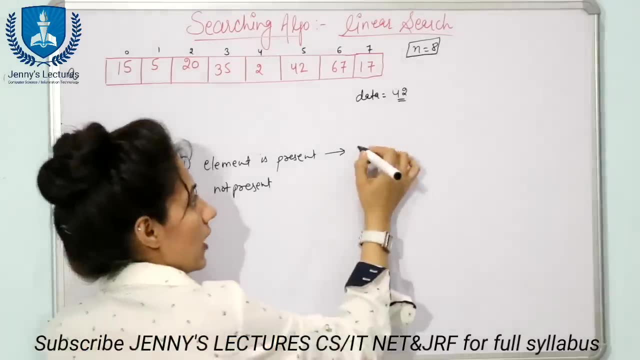 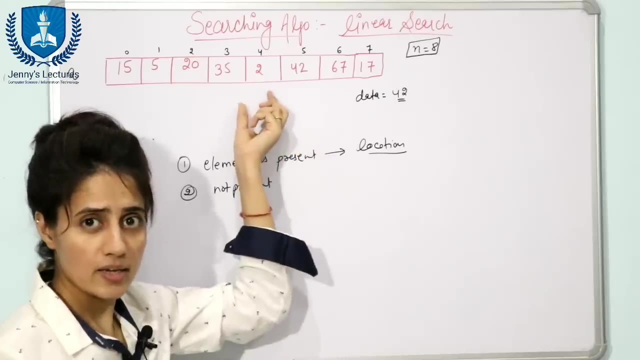 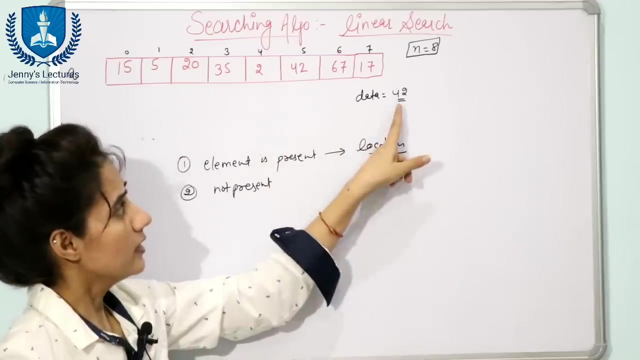 If element is present now, in that case you want to print the location of that element, where that element is present in this array. Maybe you can say at which index or you can say at which position this element is present. So see here: the index for this 42 is 5 and position is what? 6th position: 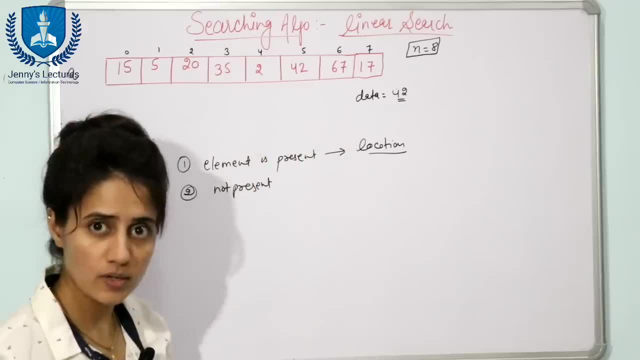 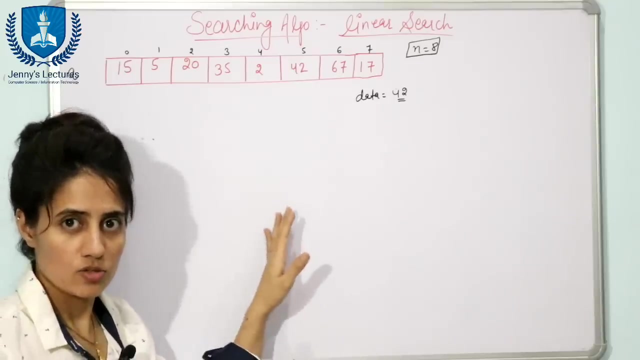 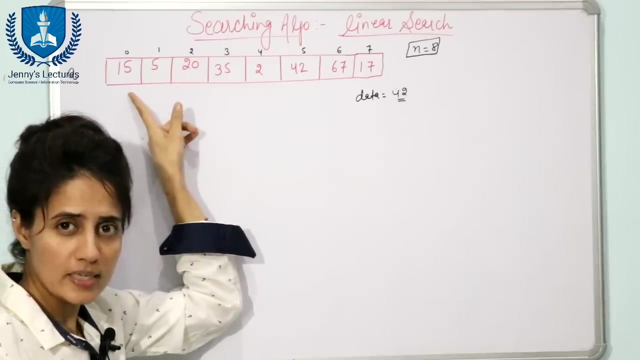 1,, 2,, 3,, 4,, 5, 6.. 6th position: Right. So either you can print index or you can print location. Now see if element is not present, then you want that your program should print element not found. So now let us discuss the working of this linear search. In this case, we are going to start our search from starting of the array, from the 0th index, Fine, And we are going to access each element of the array one by one. 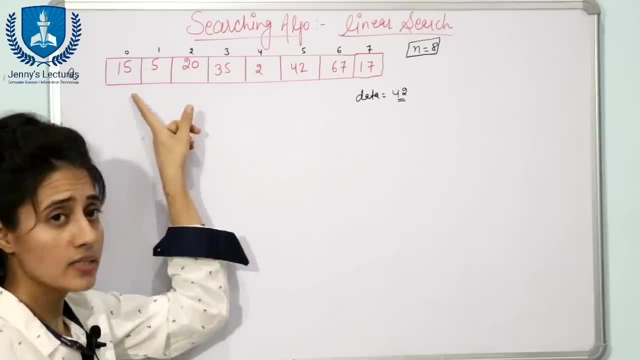 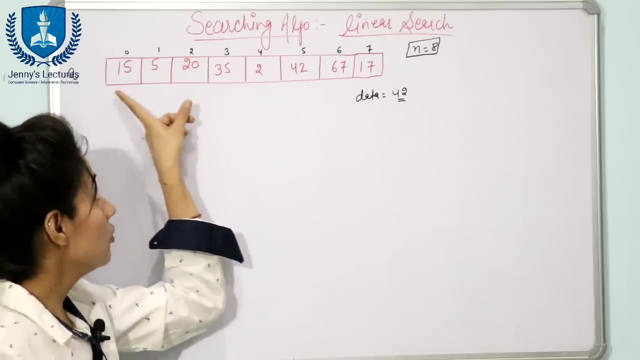 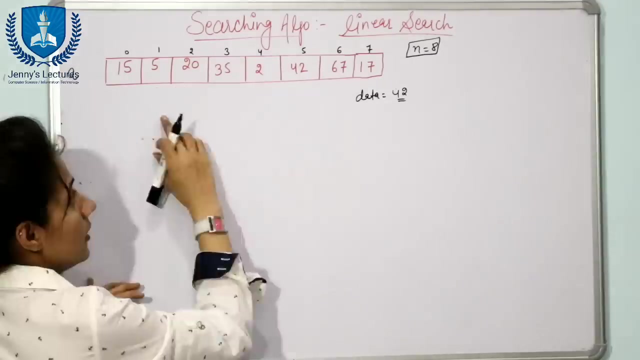 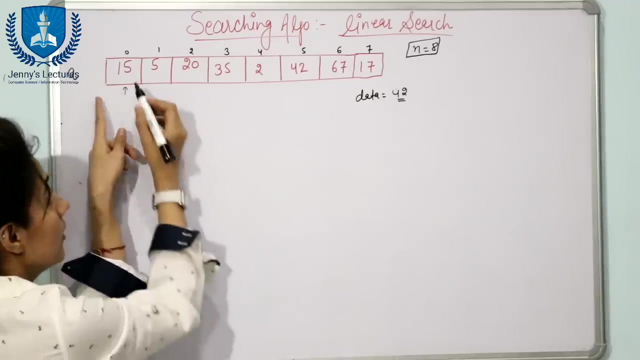 And see whether this is the desired data you want. If yes, then you are going to return that location. If no, then you are, you, you. you will move to next element, then to the next element, then next, next, next, and like this: Now see for 42. first of all, we will check here from this. we are going to start from the starting of the array 15. is this element same? you want? No, Then move to next element. 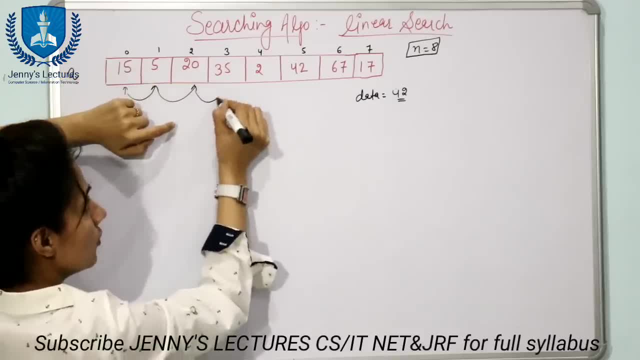 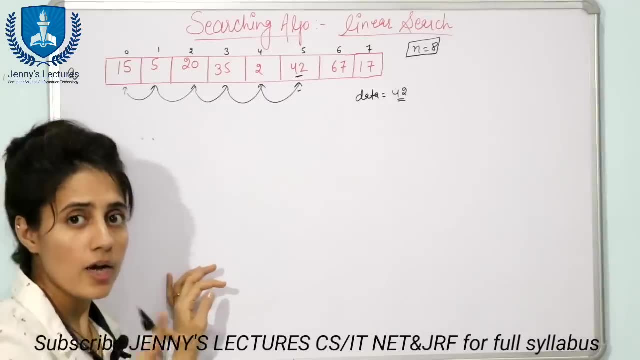 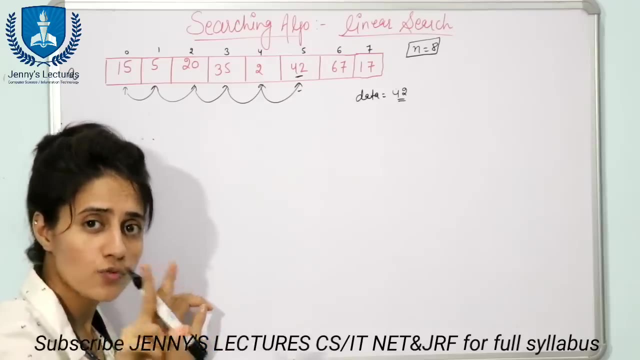 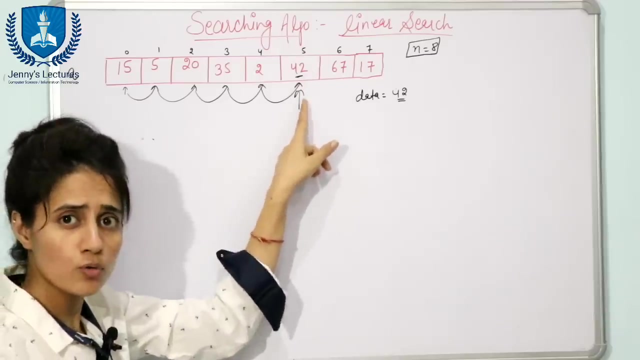 This is not 42.. Next element: This is also not 42.. This is also not 42.. Next and next: Now, here you find what 42.. Now, where you are going to stop your search, Two cases are there. First cases, first stopping condition is: you found the element Like 42. You have found the 42 here. Now we are going to stop your search algorithm here And now what this? this algorithm will return. 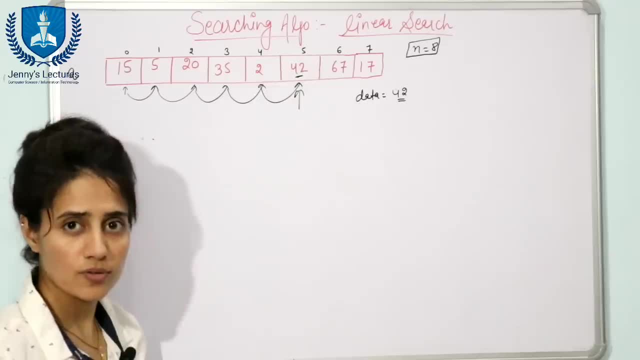 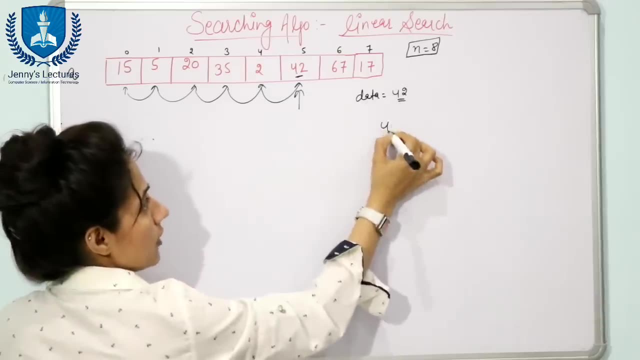 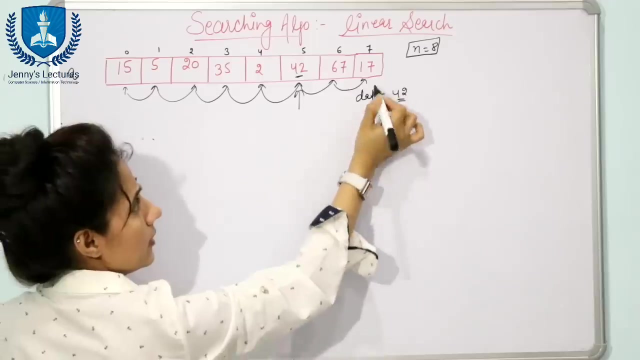 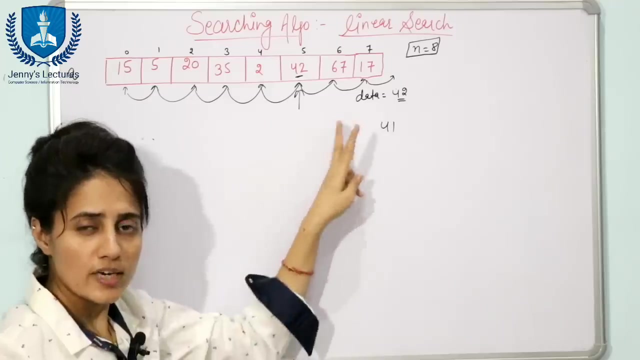 The index 5. That 42 is present at index 5.. Or second case is if data is not present in the array, Let us suppose you want to search 41. Now here is not 41. Here, not 41. Not 41. Now next. next is what You are going to stop here, Because next we don't have any element. So now, second stopping condition is you have reached to the end of the array. 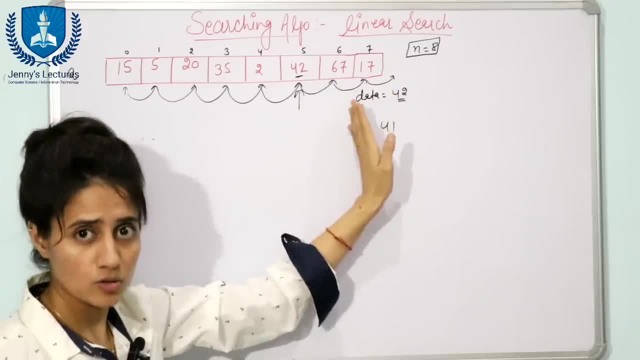 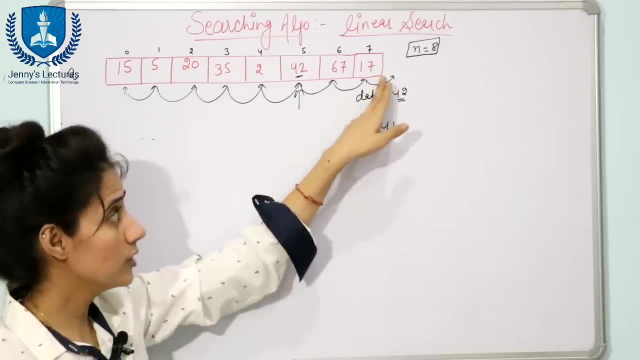 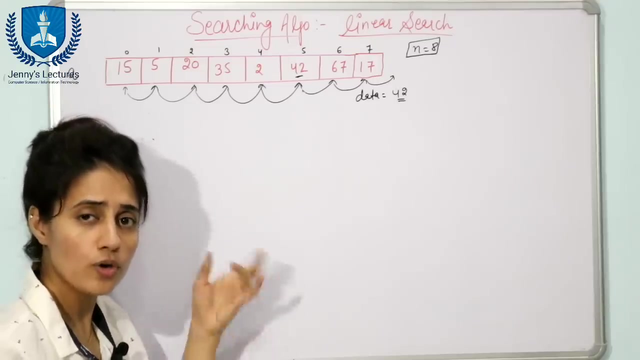 Fine, And the data is not present here. So now you have to stop. Two stopping conditions are there. Either you find the data or you reached till end of the array. Now, how to write down the code for this? See, you can. you can write down the iterative method using for loop, or you can write down a function of linear search and you can call that function in your main function. Either method you can follow. Fine, I am going to follow here the iterative approach. I am going to write the for loop, See. 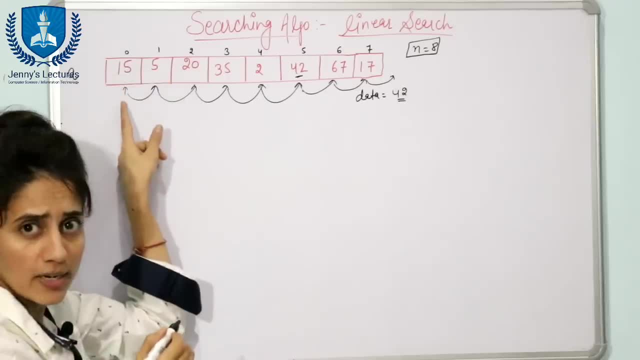 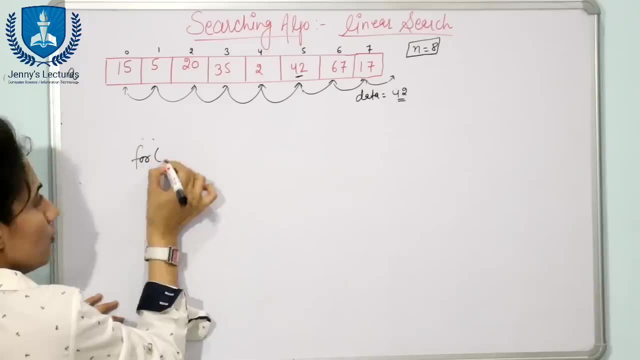 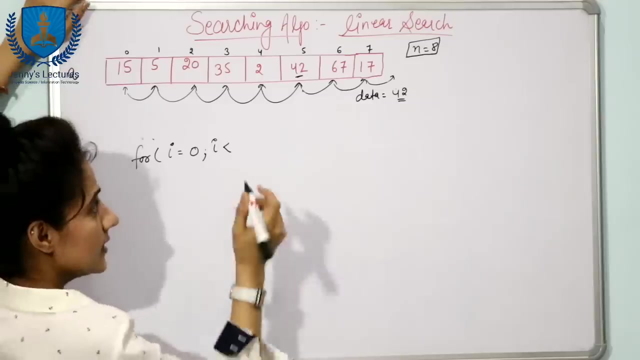 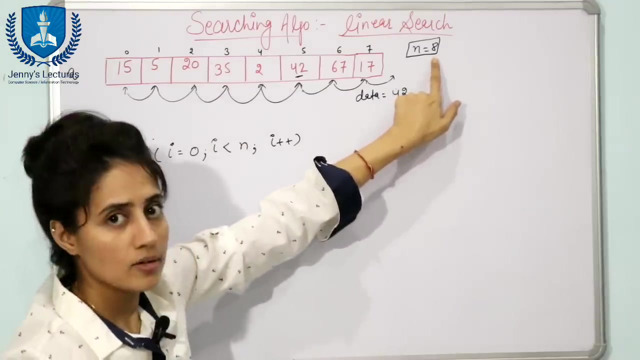 We are going to start a loop from this index, 0th index, And the loop will go till end. Right Now, see, here we have one for loop. We will take one variable: i. i is equal to starting from 0. And i less than n, And i plus plus, Because here n is 8.. So it should go till 7.. Less than 8. That is, from 0 to 7.. 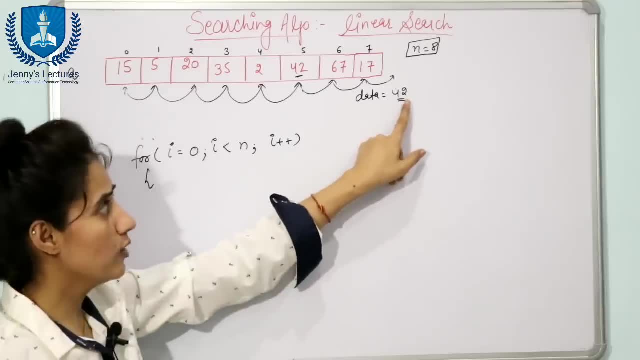 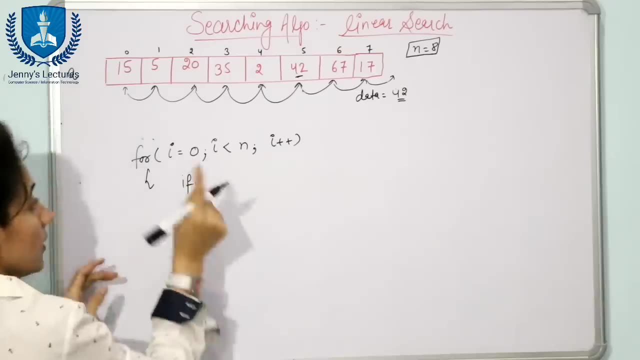 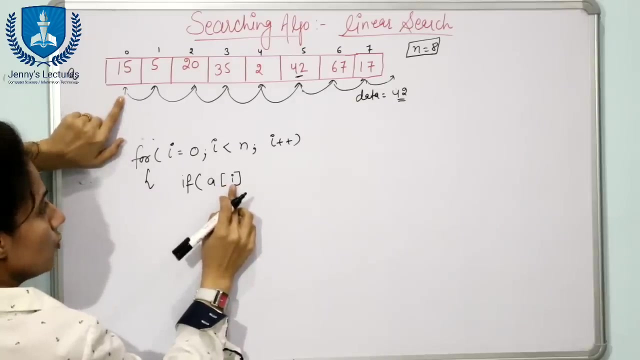 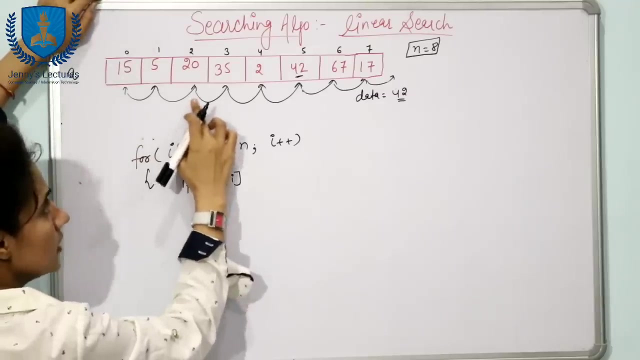 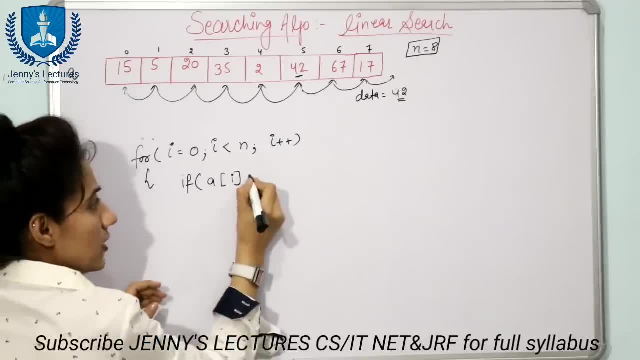 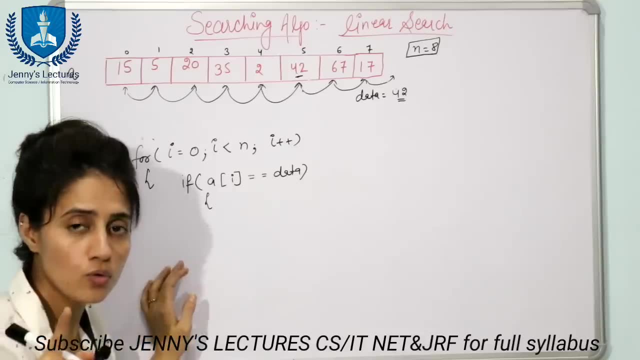 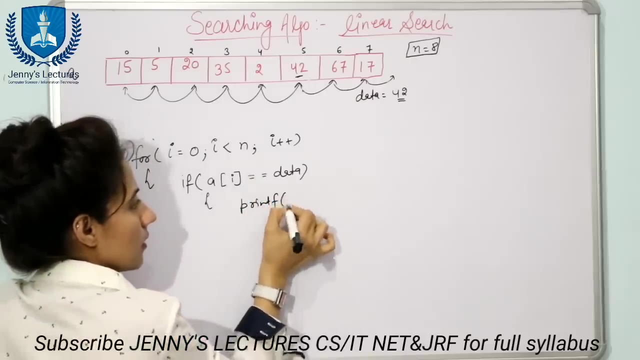 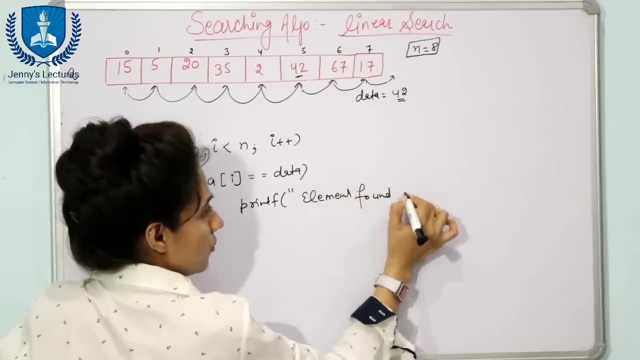 This data we want to search, Right? So if array of i is equal to equal to data, Then what you will do, You will return the location of that data, You will print. So here you will print Printf. You can write here: element found at index. 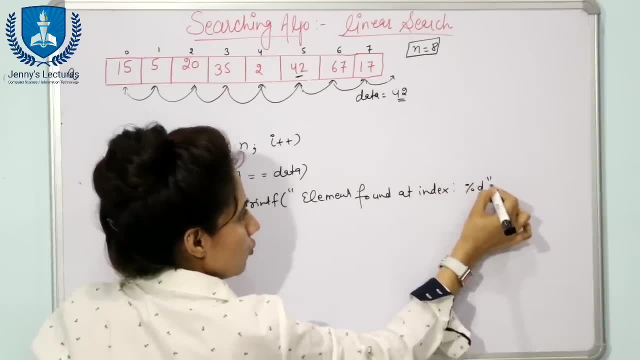 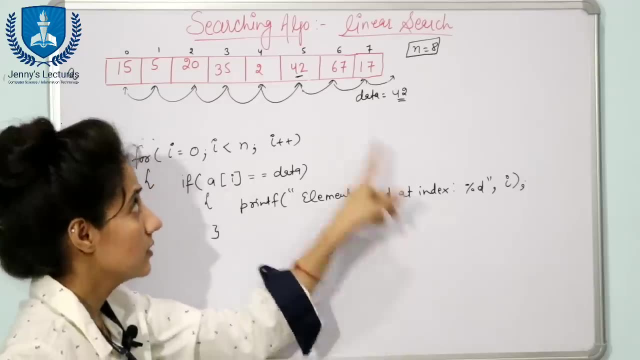 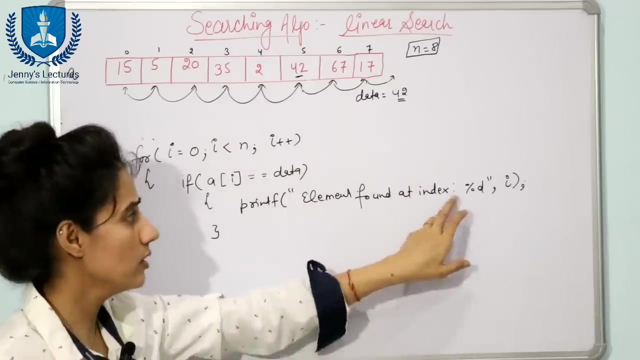 percentage d and you want to print the index, so here you will print what i right at index. so 42 would present at index. fifth, if you want to print the position, you can say: element found at position i plus one means at which position? sixth position: now suppose you are going to write. 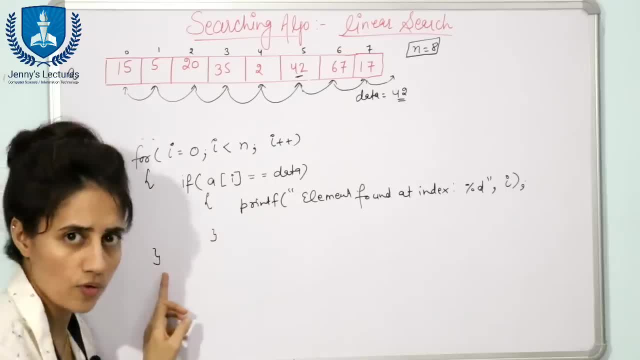 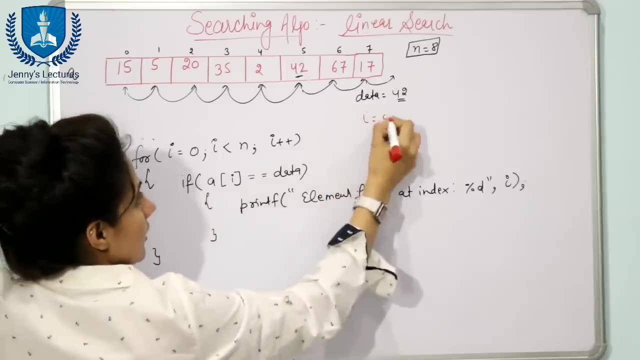 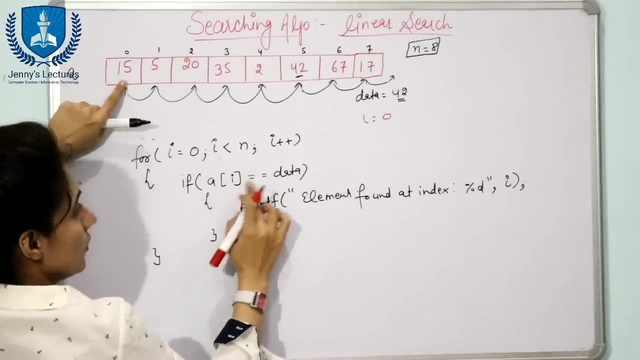 this thing. only this is closing of this. if this is closing of this four, now see, let us trace out this code with: for this 42: fine, i value is at starting. i value is zero. i is less than eight. yes, we will enter into this loop. if a of i a of zero, a of zero is 15. 15 is equal to data. data is. 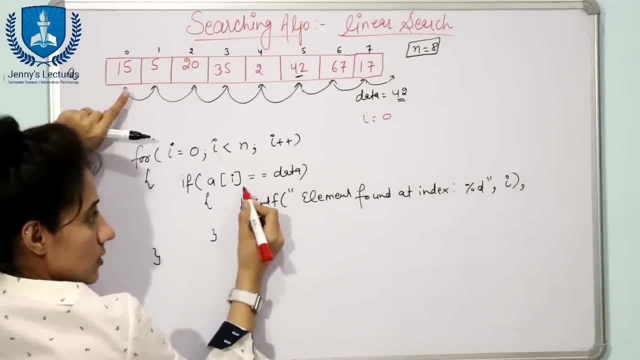 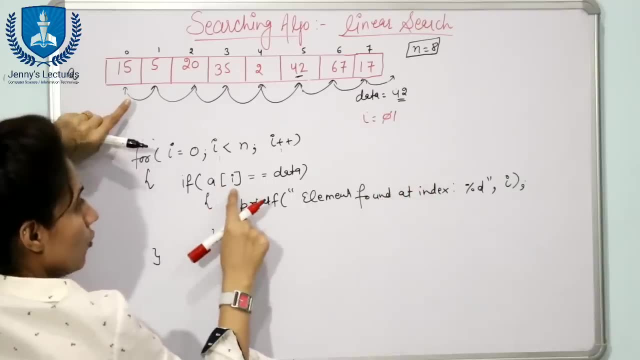 42: no, so control will not go within this if statement now, after if this: if the control will go to: i plus plus: now i is equal to one. a of one is equal to data. no, now i is equal to two. a of two is equal to data. no, i is equal to two. a of two is equal to data. no, i is equal to two. a of two is. 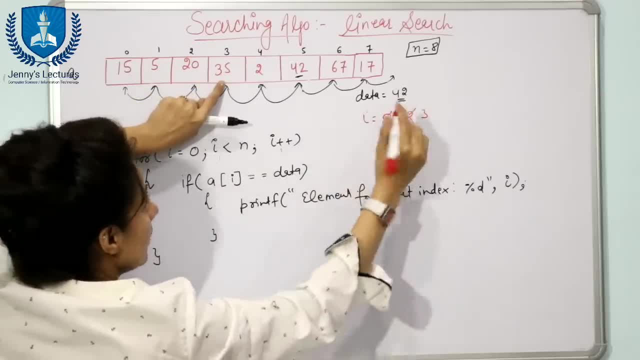 equal to two. a of two is equal to data. no, i is equal to two. a of two is equal to two. a of two is equal to three. a of three is equal to this data. no, i is equal to four. a of four is equal to data. 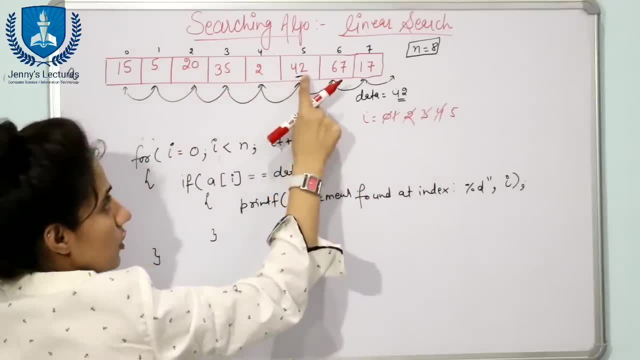 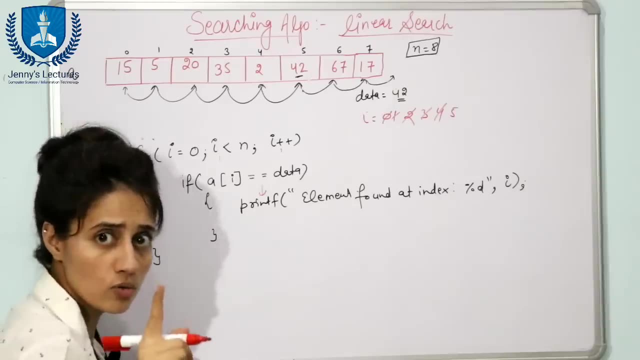 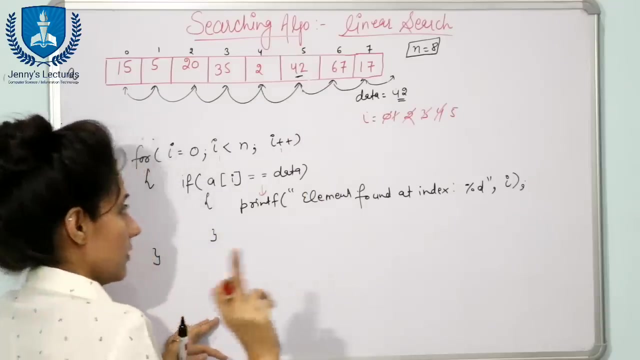 no a of five. now see a of five. a of five is 42. 42 equal to data is 42. yes, now control will go within this loop. now, what control will print? element found at index five. fine, now see, the problem is here. now see again after this: if control will go to i plus plus, now i is equal to. 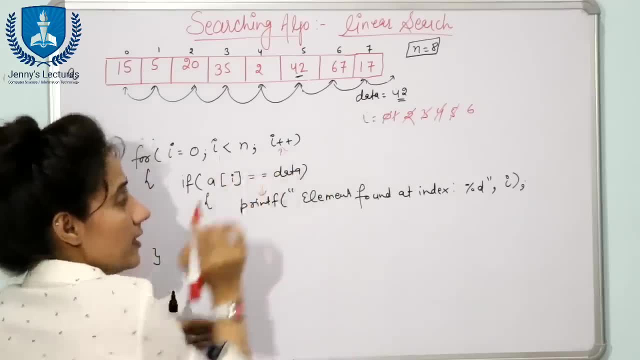 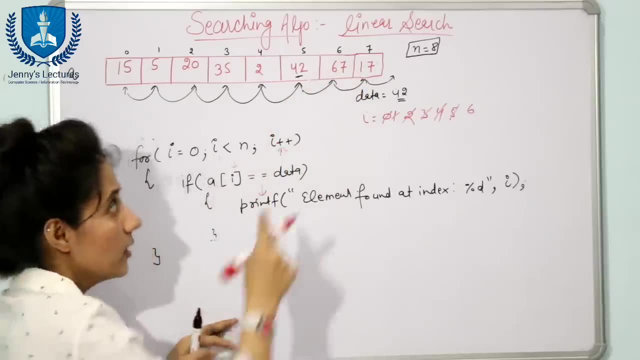 this loop. now control will go to i plus plus. now control will go to i plus plus six, and six is less than eight. right now, again, we are going to check if a of six, a of six, is equal to data. right, but that is not true. again, i plus plus i is equal to. 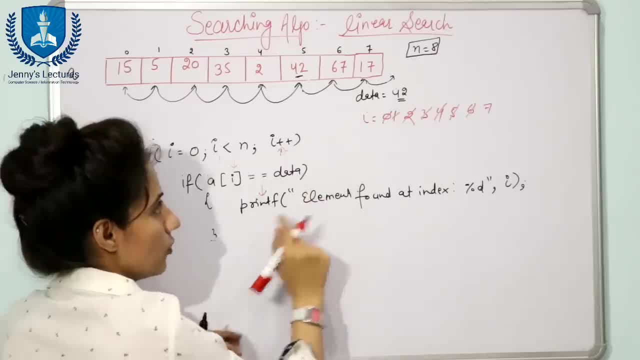 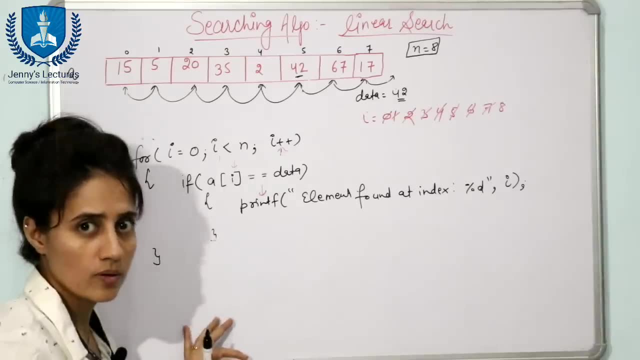 seven, again seven. a of seven, equal to data. no, we are not going to enter into this loop. now again is equal to eight. now eight, less than eight. no, now control will go out from this. for loop, now here. the drawback is what for this? for drawback is what we have found, the element. 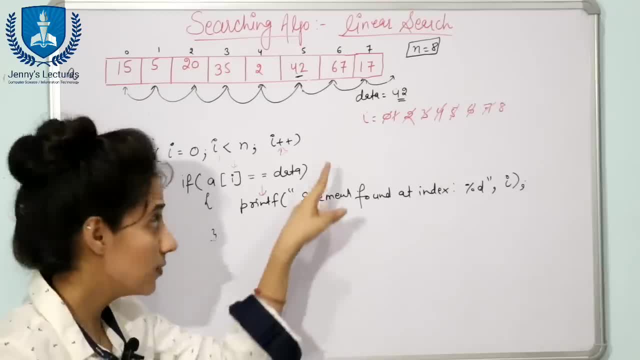 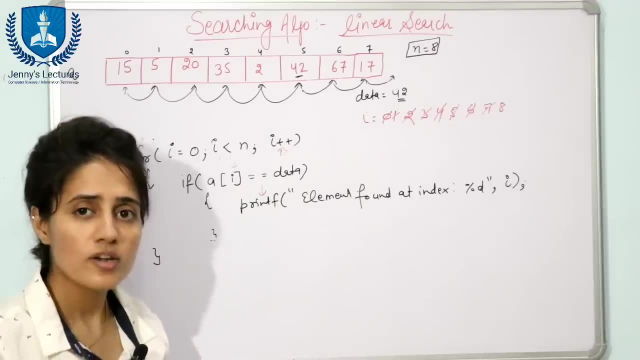 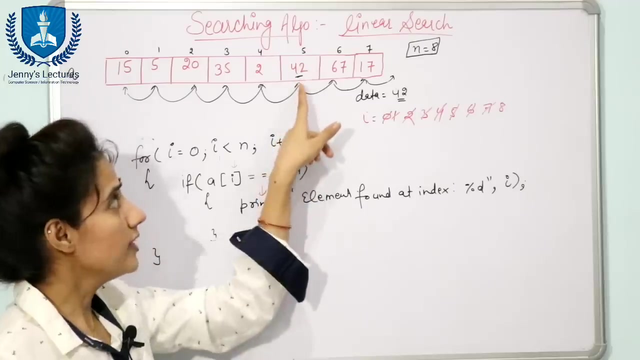 at index 5th, but still still this. this code is searching for 6th location also and for 7th index also. now what is the point to search after finding the data right? we have. we have found the data now at 5th index only. we have found 42. now, what should be done? this, this, this algorithm or 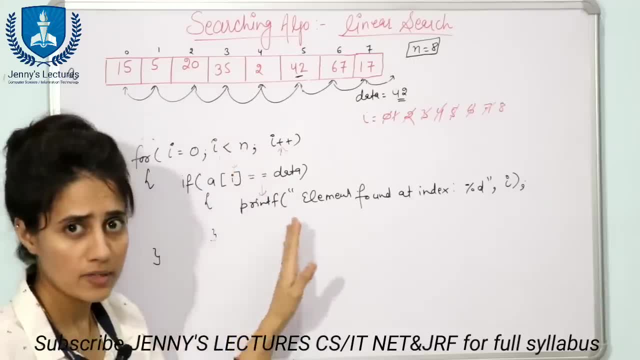 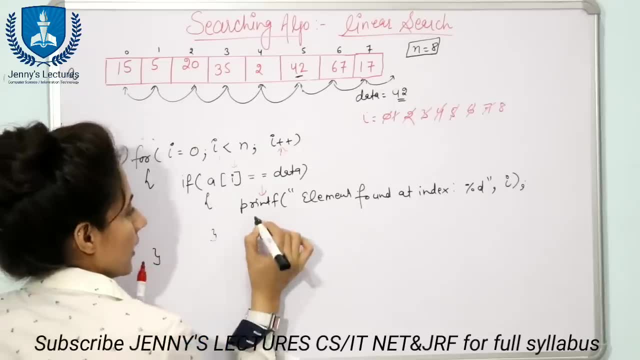 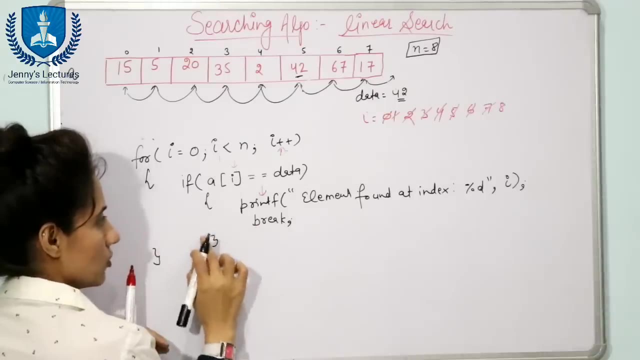 this code should have stopped at here only, but this is not stopping now. you have to add one more condition here. right, you have to write what break? after this printf, you will write break and after you will close this. if statement now see this break means what: as soon as control will. 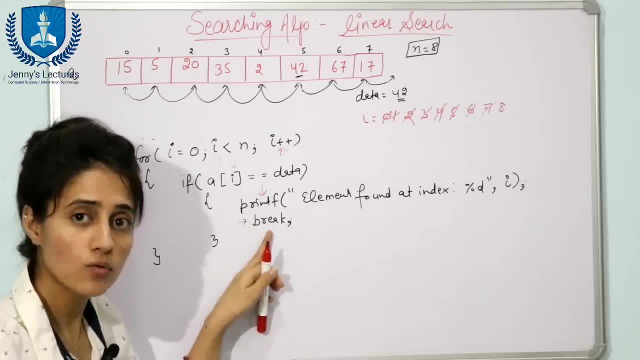 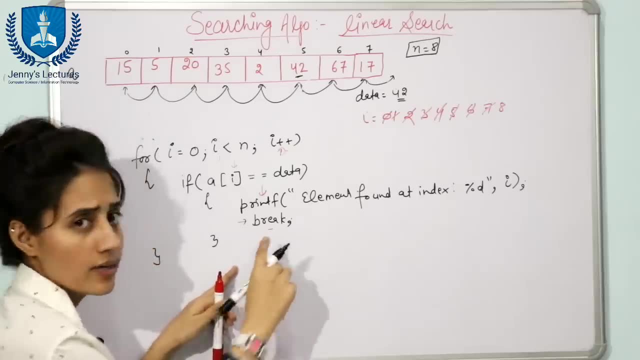 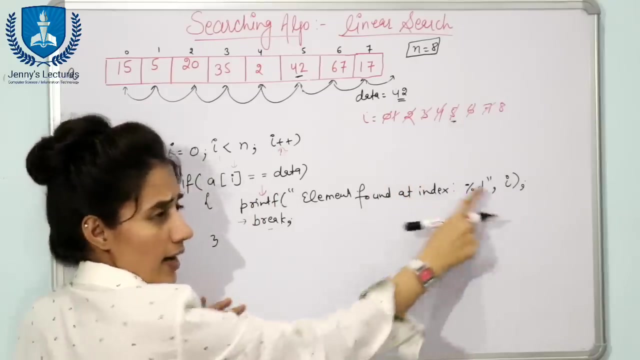 go to this break statement, then then what? the control will go out from the loop in which break statement is written. now it break statement is written in which loop which for loop here. so we found the data at index 5, at index 5, right again. control will go to here only break break. 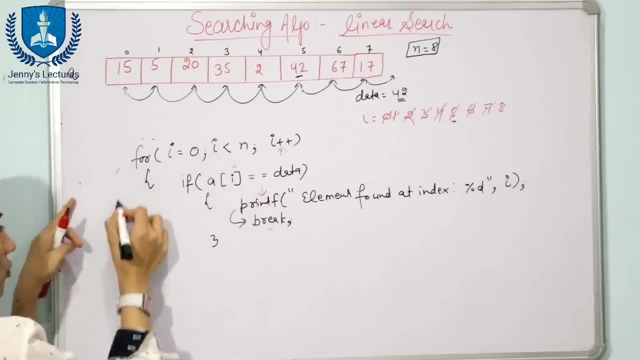 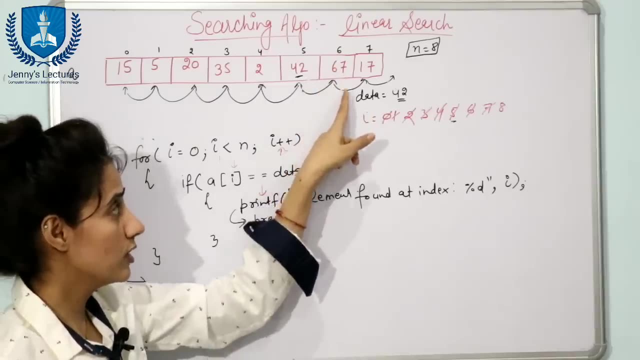 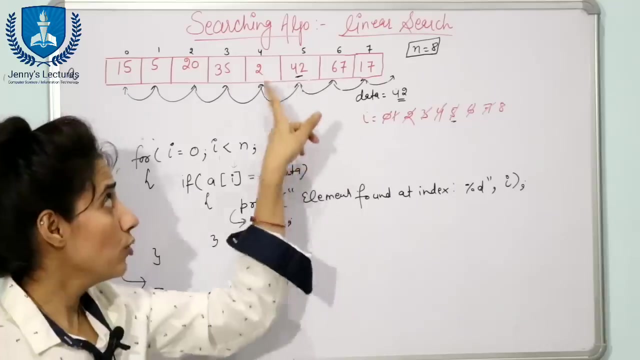 means the control will go out out from this loop, out from this loop here only now. if you write this break, then we will not search for this location and for this location. this is the stopping condition now. so now, next case is: if element is not present in the list, in the array, then what? 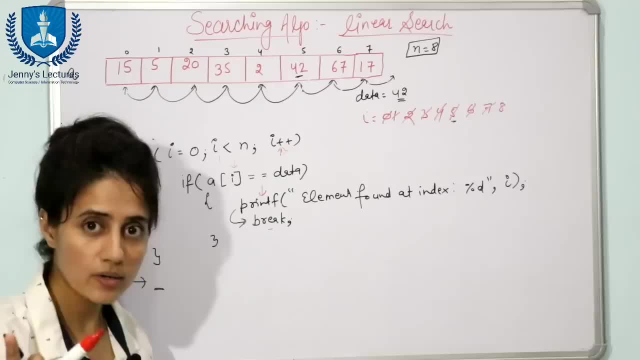 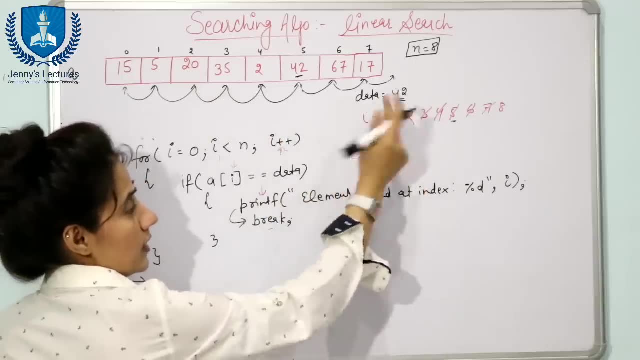 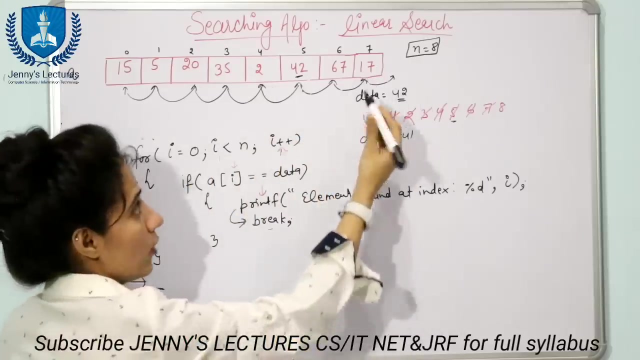 you will do. then you will print what element not found right now, where, where to write that condition, how to write that condition. see if element is not present. if suppose we are going to search data is equal to 41 and that 41 is not present now. finally, when i is equal to 7, i is equal. 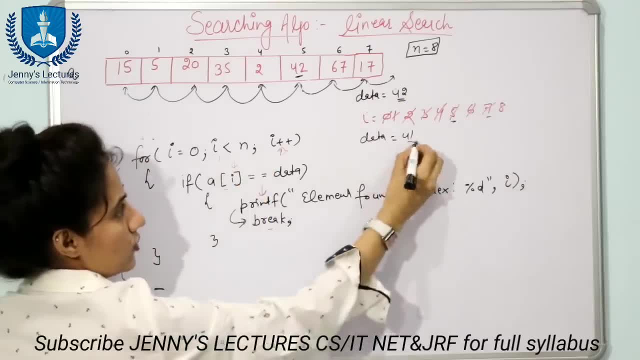 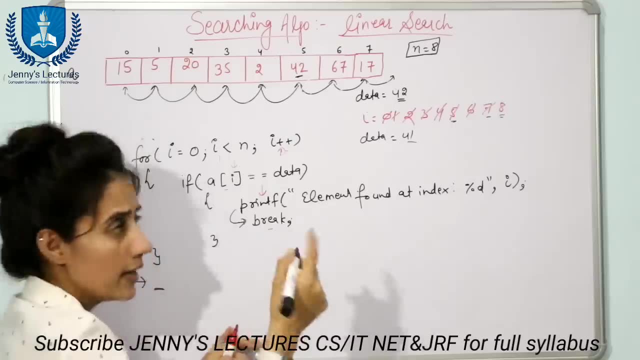 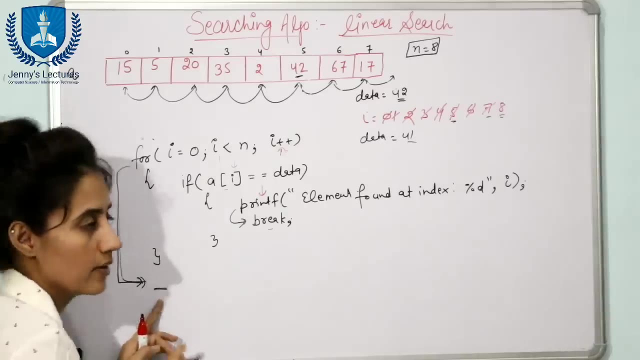 to 7. 7 is less than 8. data is 41 a of 7. is this 41? no, now again, i plus plus i is equal to i plus i plus 8, and 8 is less than 8. no, now, control will go out from this loop, whatever you will write here. 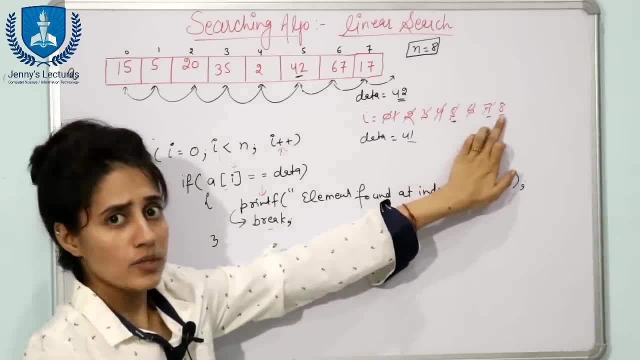 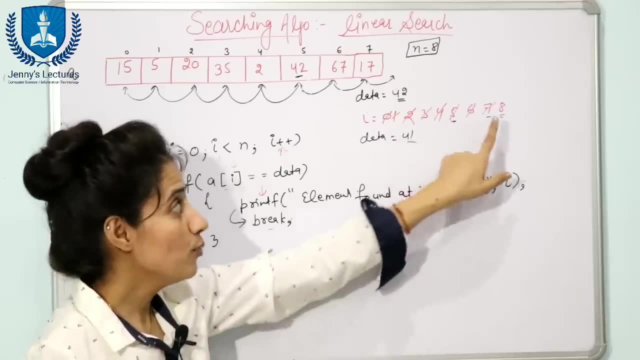 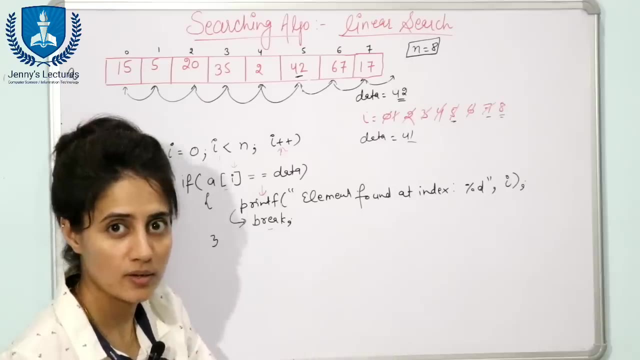 fine, it means if i value has been raised to 8. here, 8 is what number of element. it means if i value becomes same as this n value number of elements. in that case data is not present. you can say: right, so what you will write here. you will write. 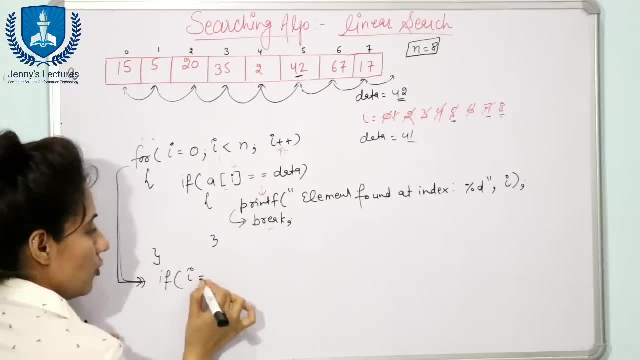 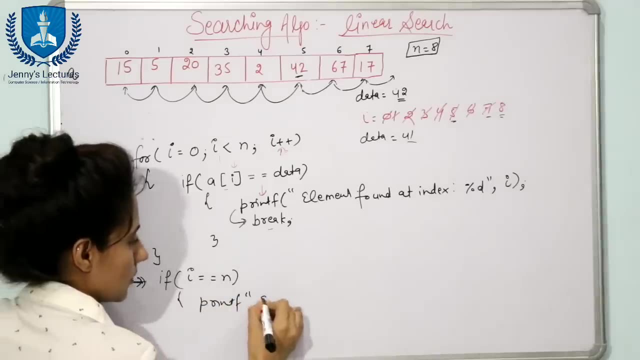 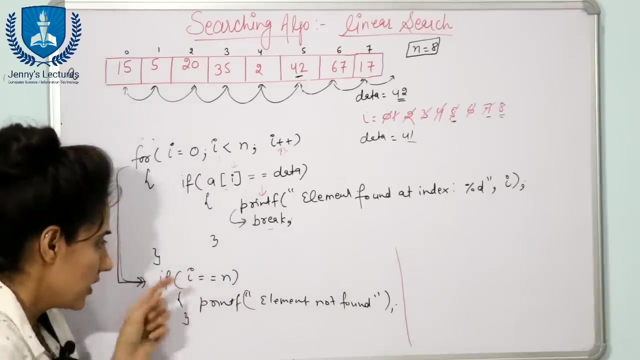 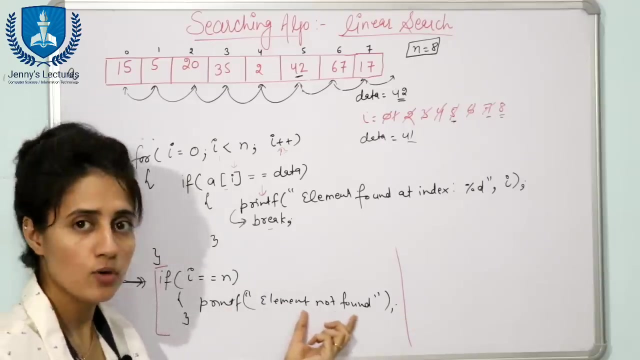 If, if i value equal to equal to n, in that case you can write here: printf: element not found. And if you don't write this condition, if you don't write this one, One second method to print this statement is: element not found is c. 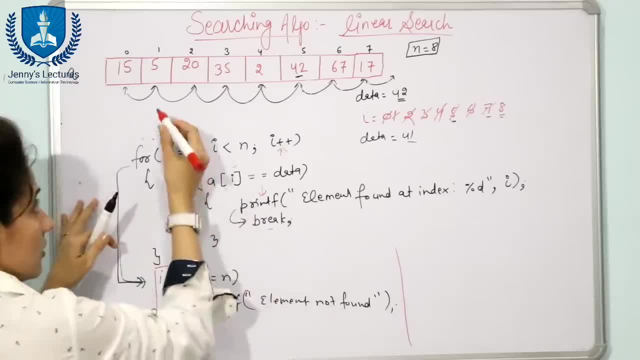 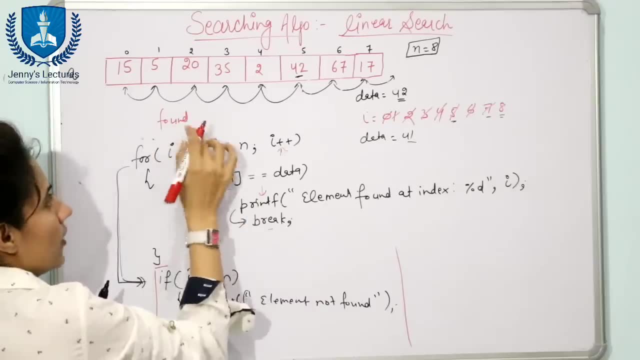 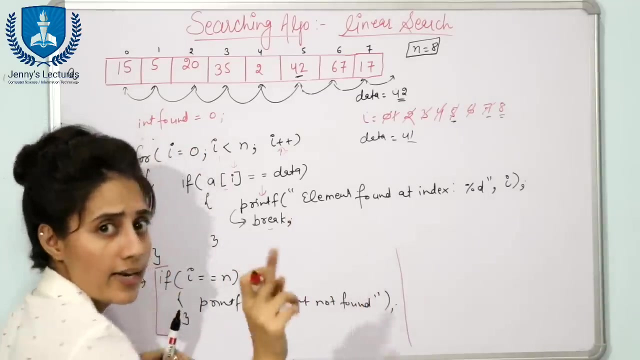 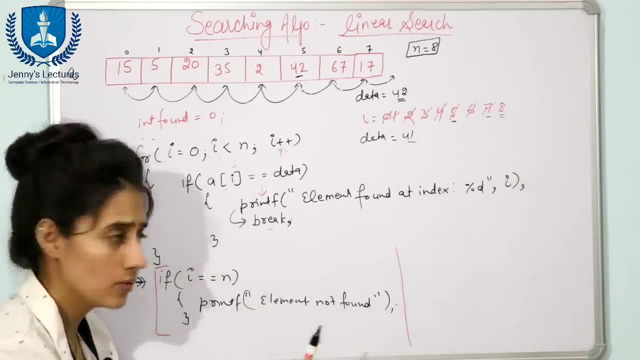 You can take one variable here at the starting. you can take either found or flag, it's up to you. I am taking found, a variable. found is equal to 0 in the program at starting And if you find the element, in that case you will do what you will. you will convert this found value to 1 means found is equal to true. now we have found the element, right. 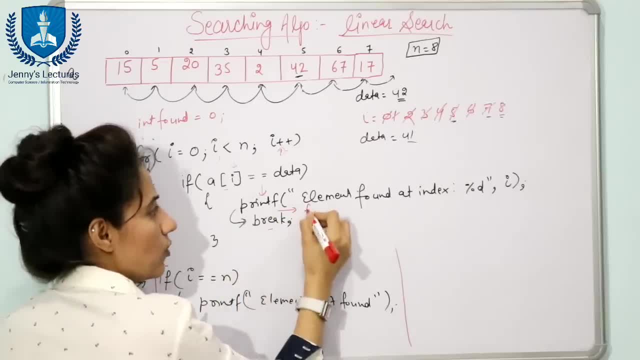 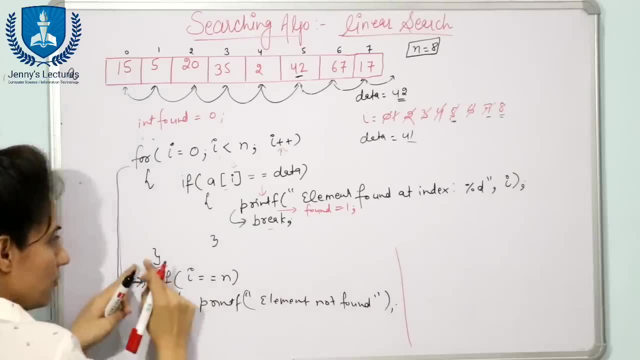 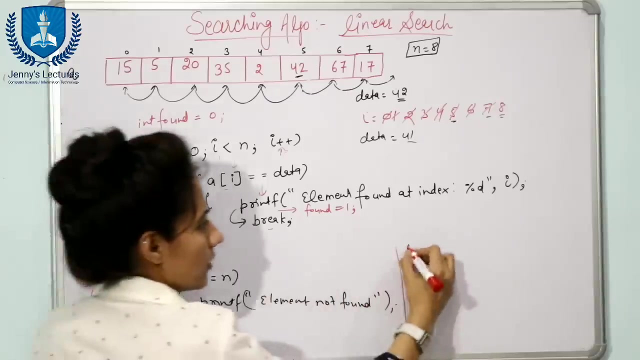 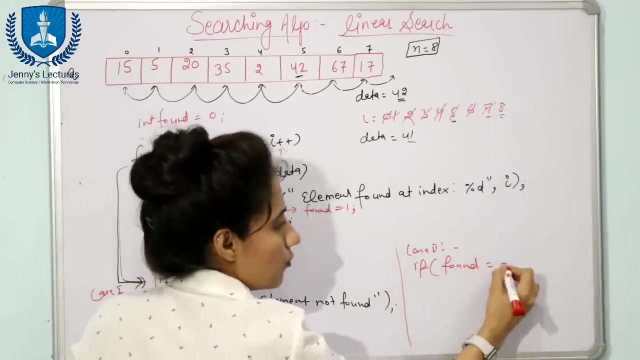 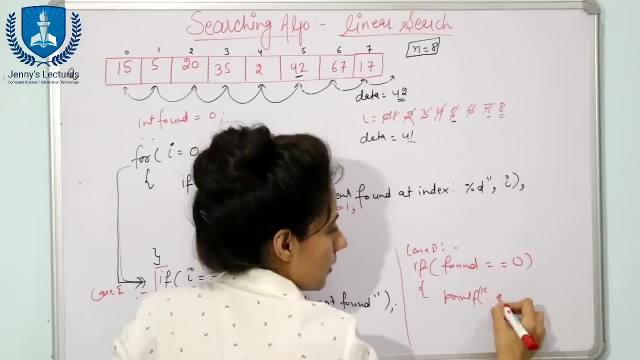 So before this break, before this break, here you will write what Found is equal to 1, right, and here after this, after this 4. if you don't write this condition, then second case is: this is case 1, you can write this also. this is case 2 and you can write this also. here you can write: if found is equal to is equal to 0, it means you can printf here: data not found. 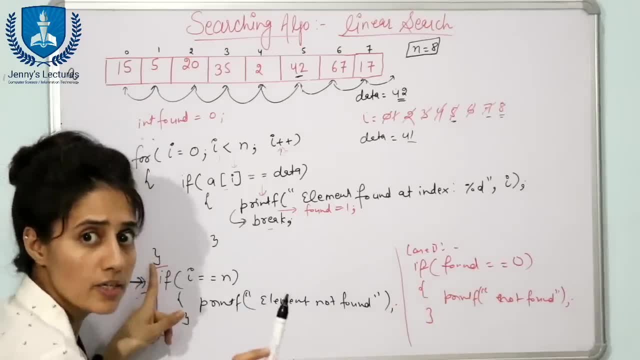 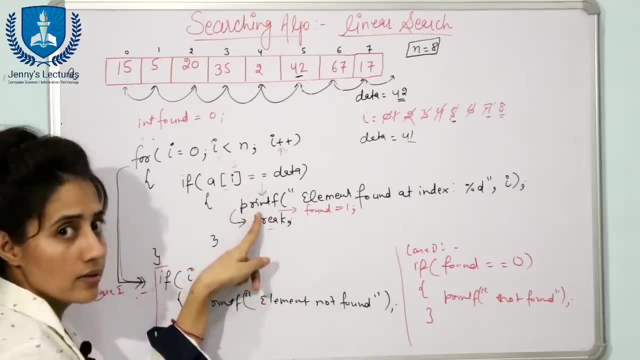 If found is equal to 0, it means it means control has not entered into this. if condition here means this condition never becomes true. so that is why. that is why after the for loop also still found is equal to 0, it means found is equal to false. element is not present, so you can write element. you can say: element not present, so you can write this also. you can write this also. 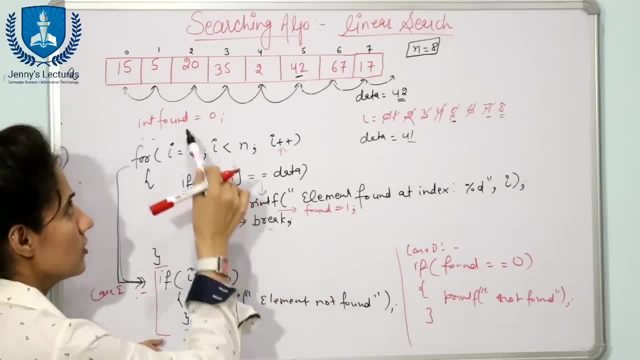 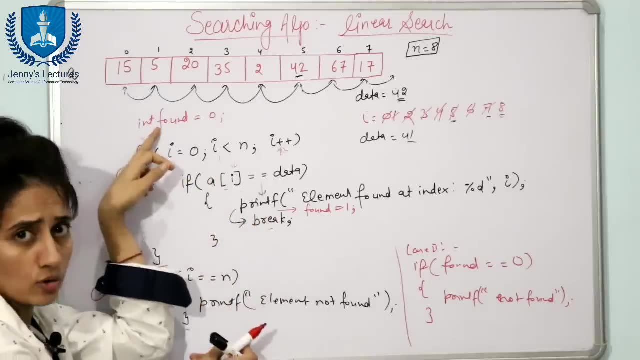 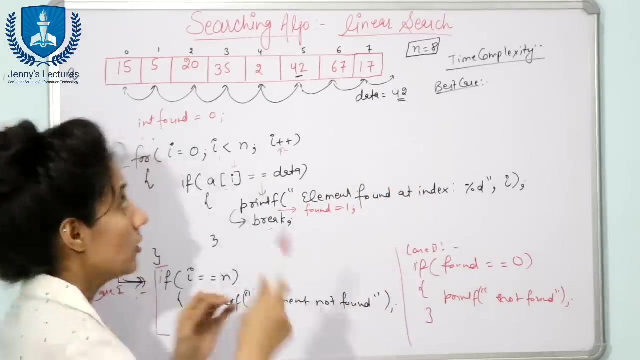 If you follow, if you write this case, then you do no need to declare this found variable. see, this is not the complete program, so you have to write some another statements. also, this is just the main logic, not the complete program. so now, what is time? complexity, first of all. we are going to check in best case. best case is what? suppose? this is our array and you want to find out? data is equal to 15.. 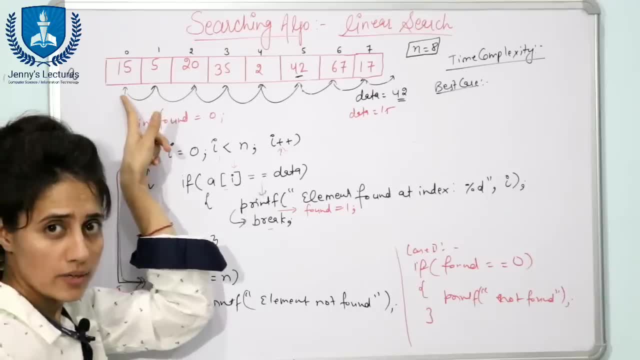 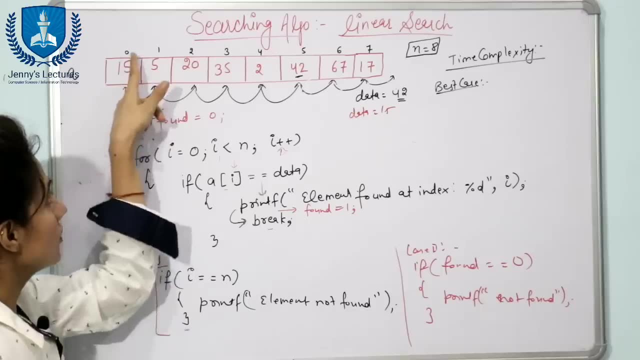 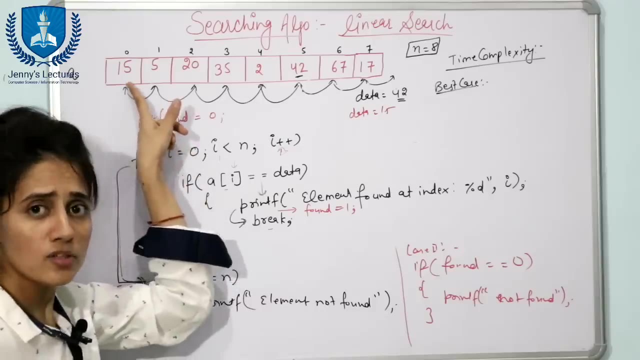 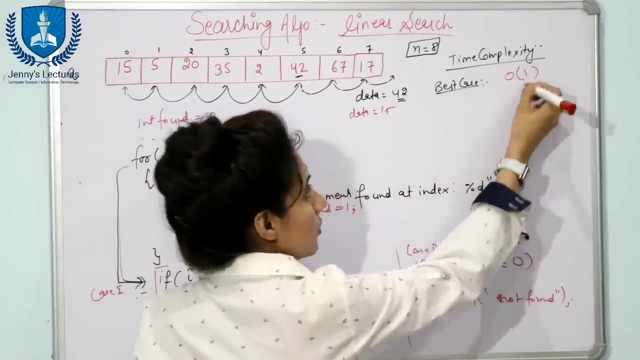 Fine, in linear search we are going to start from the initial point of the array, from the 0th index. Find out, check 15 first at first index, at 0th index we have value 15. 15 is equal to this data. yes, it means in one comparison only you have got the data. so in the best case, the time complexity would be order of 1 only. what about worst case? 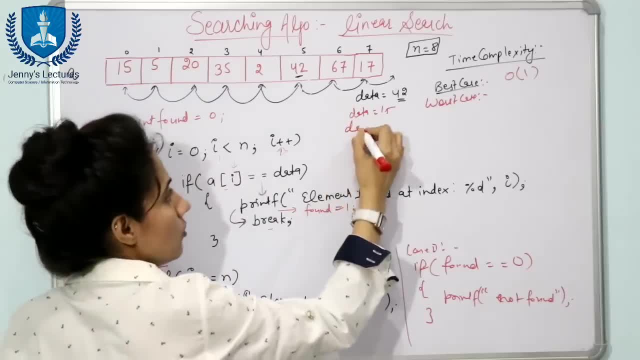 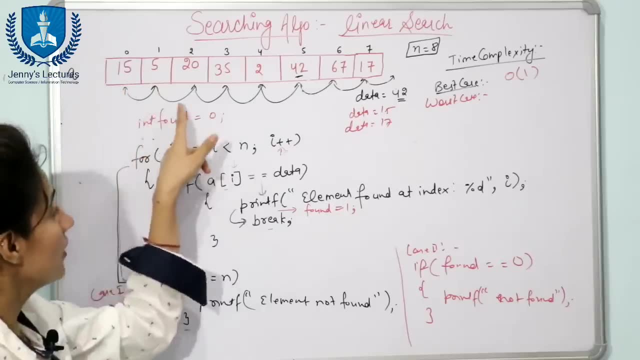 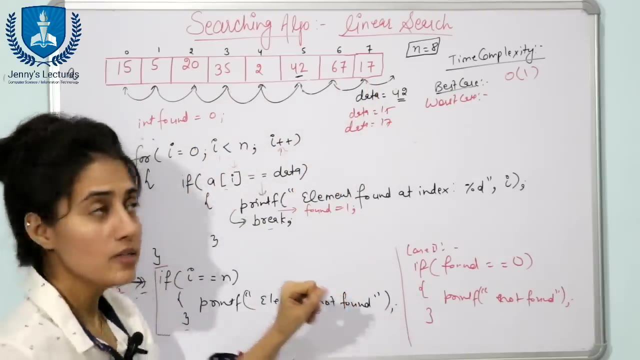 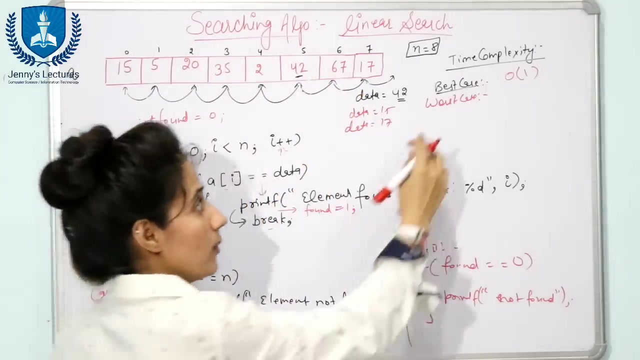 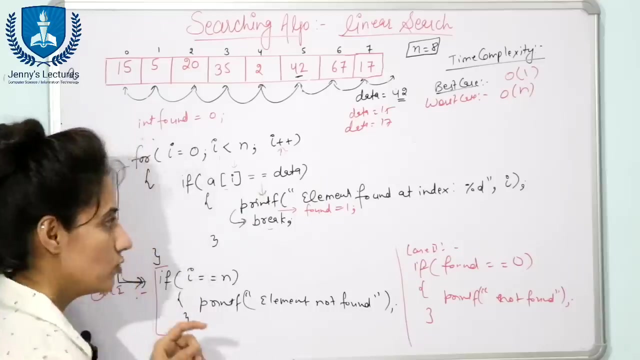 Worst case means: suppose you want to find out the data 17.. Here how many comparisons you have to do: first of all 15, then 5, then with 20, then 35, 242, 67 and then 17, and here you got the data. means n, n comparisons, 8 comparisons. right, so that is why here the time complexity in worst case is order of n. the number of elements: total number of elements: n. if you find out the time complexity, you just, you just do what: check out where is the loop.